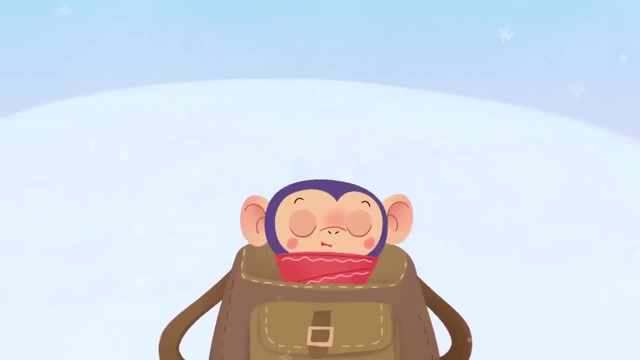 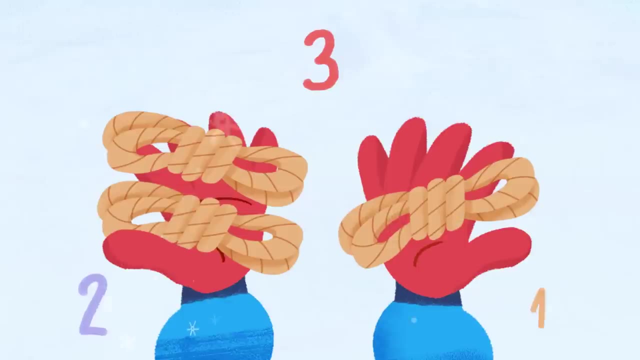 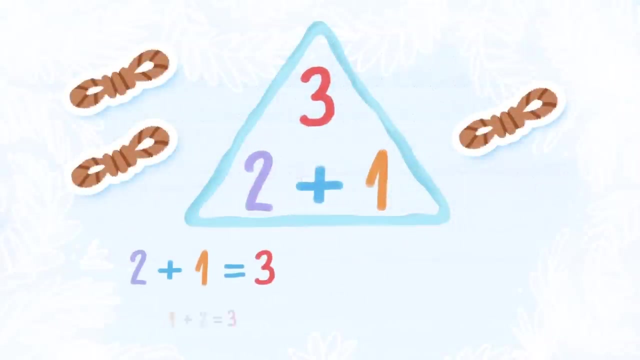 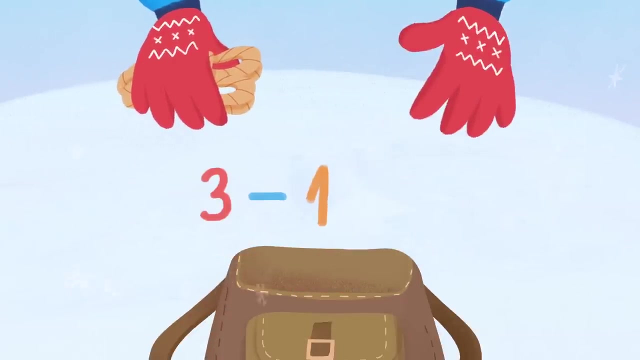 I will show you one of the most basic fact: families. So I have three ropes: Two ropes for the dog and one rope for the sled. Let's see: Two plus one is three, And one plus two is three. I can keep this rope in my pack. So three minus one equals two, And three minus two equals one. 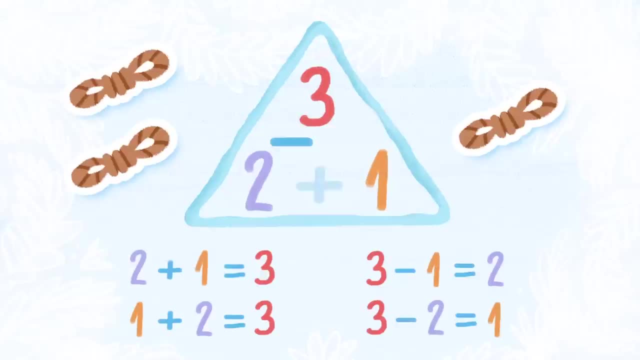 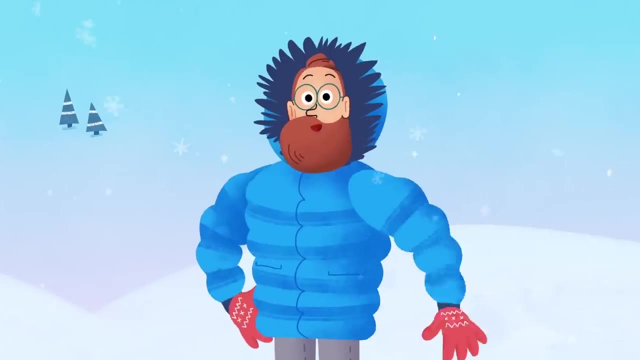 Now I have one rope in my pack and two for the dogs. That's a fact, family. Here are our sled dogs. Before we go for a sled ride, I'm gonna give them a treat. Look what I got for them: Fresh fish. 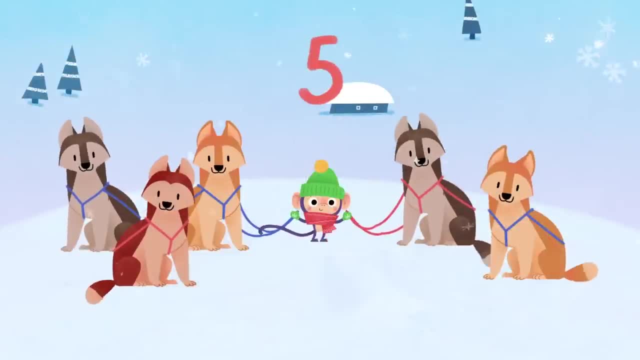 So there are five sled dogs: Three dogs on this side and two dogs on the other side. So there are five sled dogs, Three dogs on this side and two dogs on the other side. So there are five sled dogs, Three dogs on this side and two dogs on the other side. 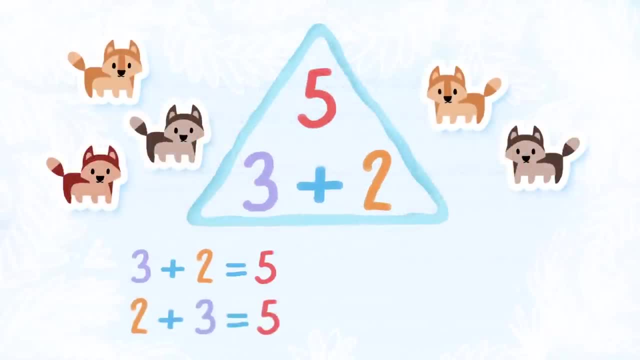 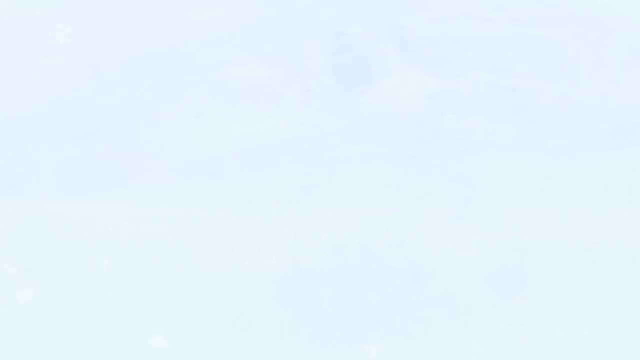 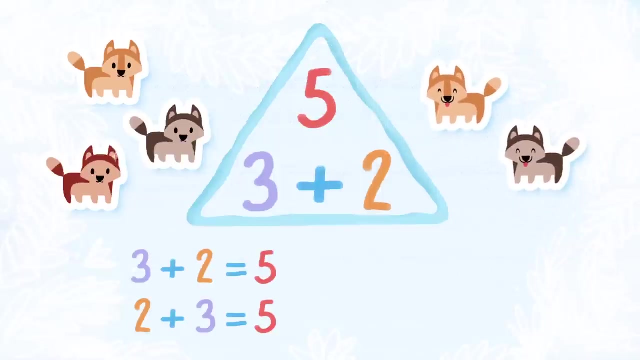 Three plus two is five. Two plus three is also five. Let's unleash two dogs so they can come and get a treat. So far I've given two dogs a treat. How many more dogs need a treat? Five minus two is three. That's right. 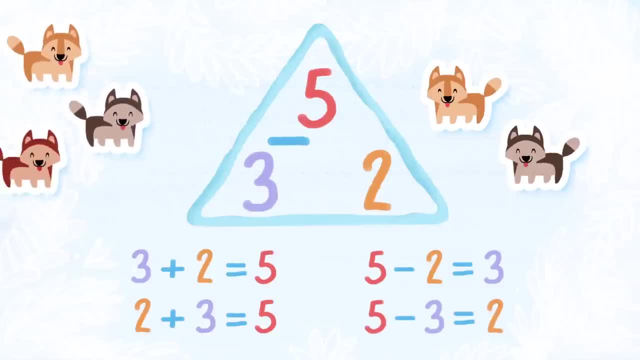 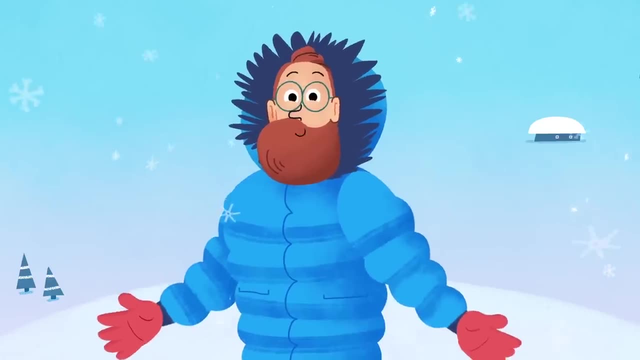 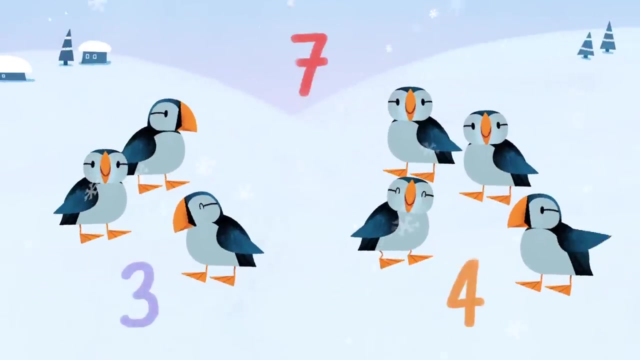 And five minus three gives us two. That's the whole fact family. Finally, the dogs are ready for the sled ride. Let me show you some more fact families. Look at those lovely birds. Do you recognize a fact family? Three plus four is seven. 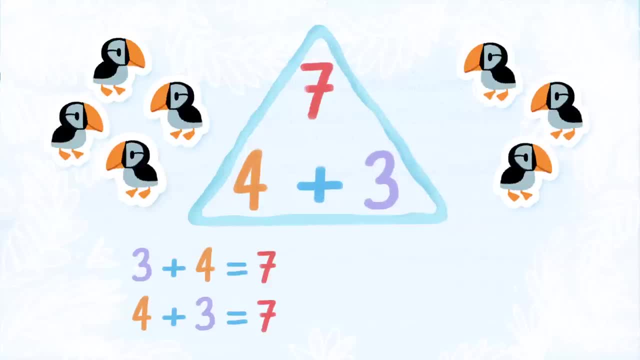 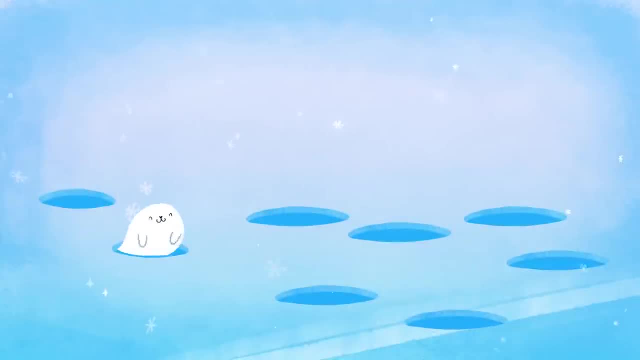 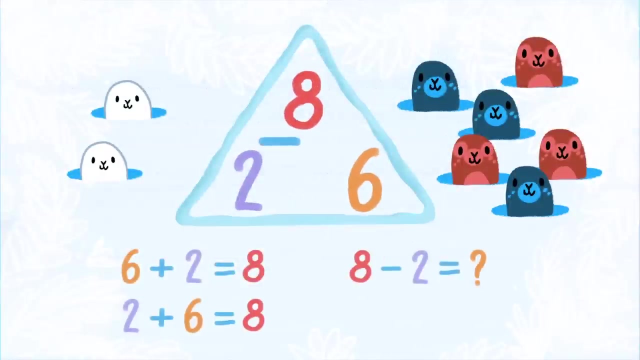 And four plus three is seven. So seven minus four is three And seven minus three is four. Perfect, Look at those cute baby seals. Six plus two equals eight. Two plus six equals eight. So eight minus two equals six. That's right.